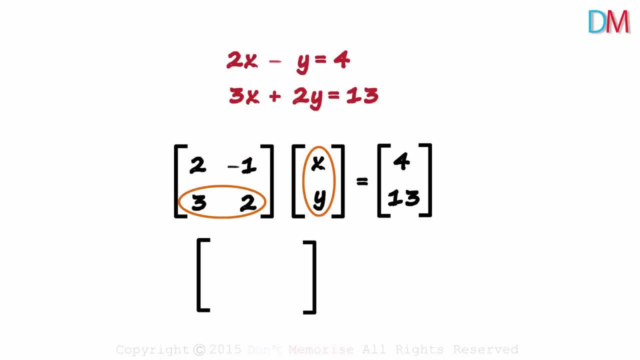 What will be the product of these two? It will be 2x minus y, And the product of these two will be 3x plus 2y. This is the product of these two matrices, And this matrix will be written as is. 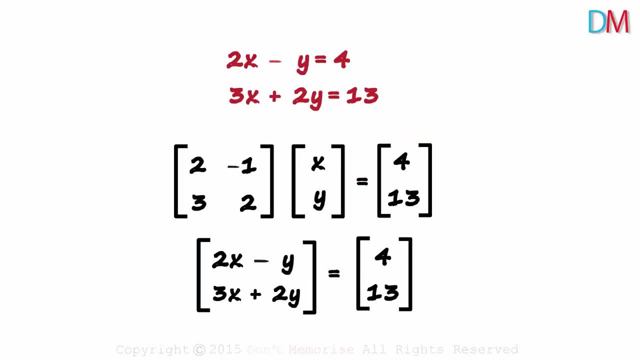 Now you see why this is the matrix form of the system of equations. As these two matrices are equal, we can say that 2x minus y is equal to 2x plus 2y. This will be the product of these matrices. 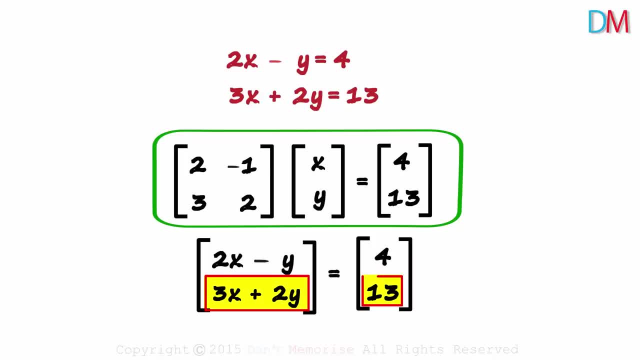 will equal 4, and 3x plus 2y will equal 13.. Same as these two equations. But let's come back to the important point. How does writing it in matrix form help us solve the equations? Let's see that on the right hand side. 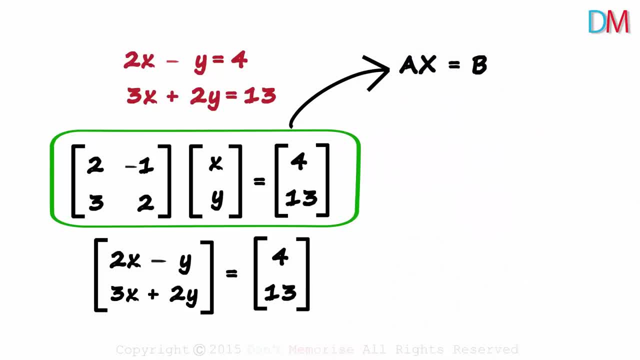 This can be written as: A times X is equal to B. We have called this one matrix A and this matrix X and this matrix B. A times X is equal to B. What we're interested in is matrix X. That will give us the values of variables X and Y. 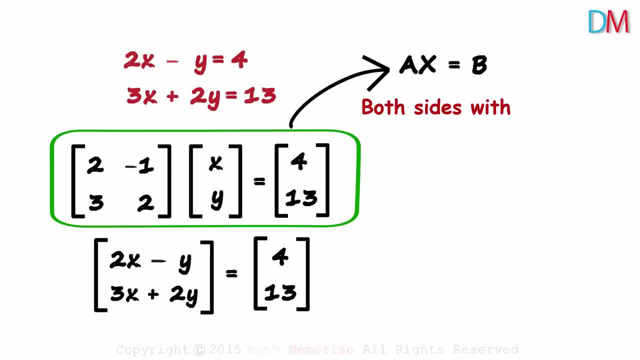 So to get X on the left hand side, we multiply both sides with A inverse. We get the left hand side as A inverse times AX and the right hand side as A inverse times B. Now A inverse times A will equal the identity matrix. 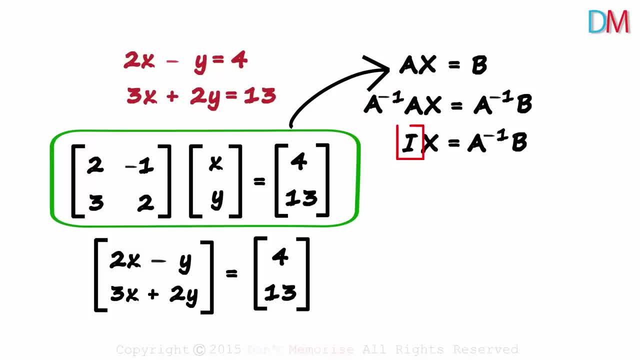 We get this And we know that the identity matrix times any matrix will give us that same matrix. So the left hand side will equal matrix X And the right hand side will be A inverse times matrix B. That's how we get matrix X. 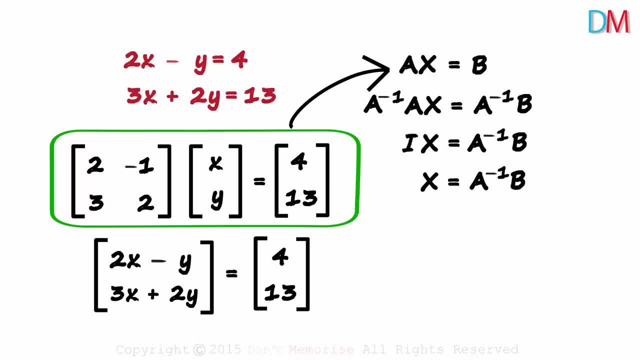 We multiply A inverse with B. So when we are given the two equations we write it in this form: Find the inverse of this matrix and multiply it with this to get matrix X And that will give us the values of the variables We will solve for the matrix. We will solve this example in the next lesson.